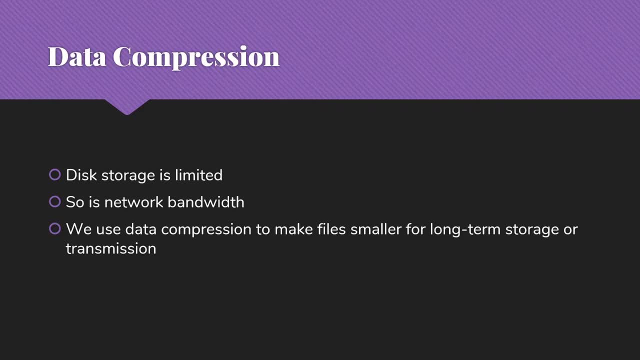 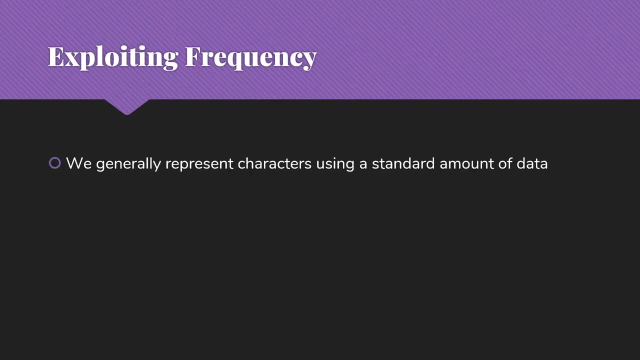 or even more frequently. we're wanting to make them smaller so that we can transmit them more efficiently. There are many approaches to compressing data. What I want to talk about today is exploiting frequency, specifically frequency differences. So when we think about how we usually represent characters, we typically are using a standard amount of data. 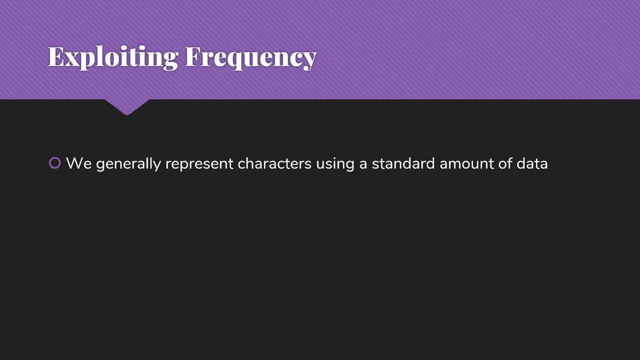 one byte, two bytes depending on our specific encoding, maybe up to four bytes, But we're pretty consistent across specific character values within a given encoding or set of characters. In most text, however, character frequencies vary widely. For example, in English, if we have much text, 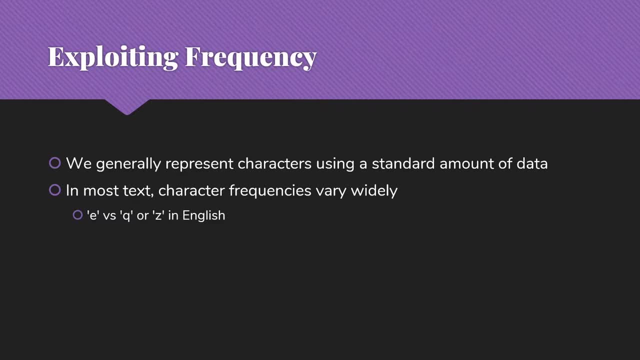 the letter E is probably very frequent. The letters Q and Z are likely to appear very little, if at all. The idea, then, is that we're going to see a lot of different types of characters, and we're going to see a lot of different types of characters. 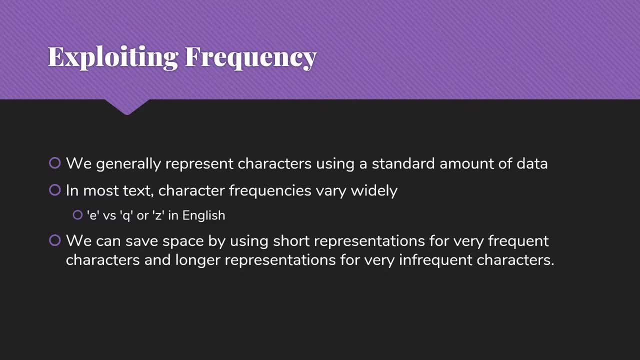 We save space by using shorter representations for very frequent characters- so example E in English- and longer representations for very infrequent characters. This is going to allow us to represent all of our different data but use less space total. We're also going to get some savings from the fact that many of our documents aren't going to use all of the possible characters. 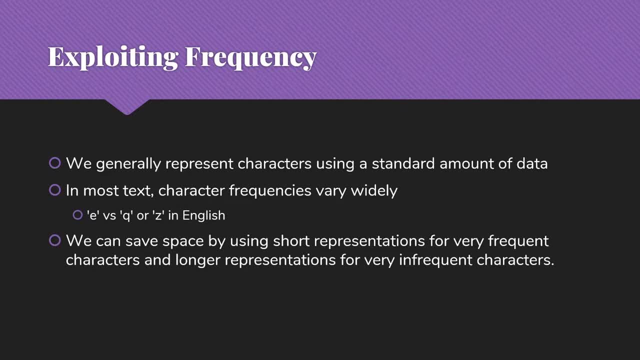 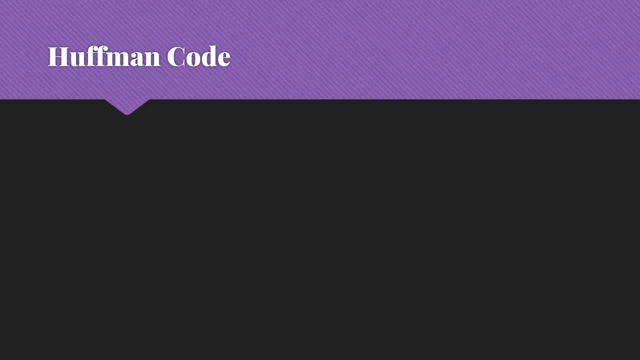 So we're going to have fewer characters to represent to start out with. Let's take a look at the second reading. So the kind of code that we're going to use is something called Huffman code. This is a specific approach to exploiting these character frequencies, which is guaranteed to be optimal. 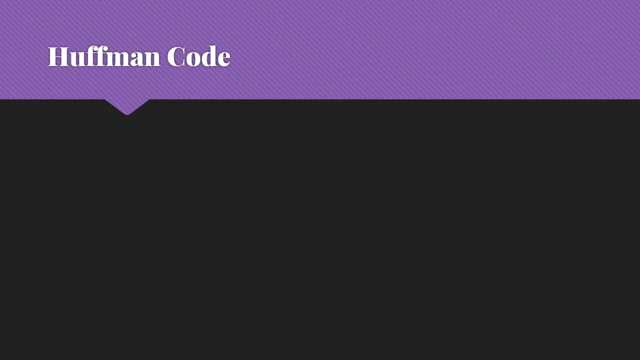 given that we're doing character frequency and handling our compression this way, It's not going to be the optimal compression for all data, But it will be the optimal compression for this approach to compressing the data. The idea here is we're going to first read the file to be compressed and just count. 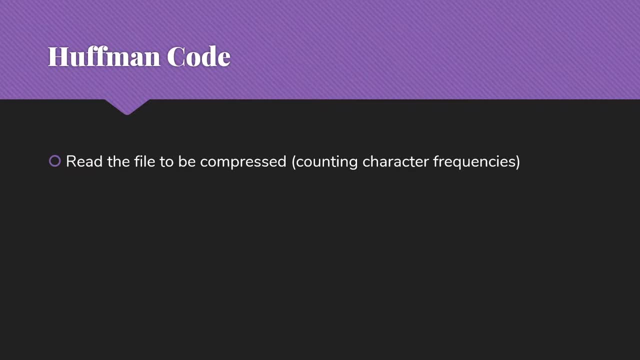 character frequencies so that we know here are the characters that show up in our file and this is how frequently each of them shows up. Once we have that information, we're going to produce the optimal code with variable length encodings based on that frequency, and, of course, we'll go into much more detail about how we do that Once we have that code. 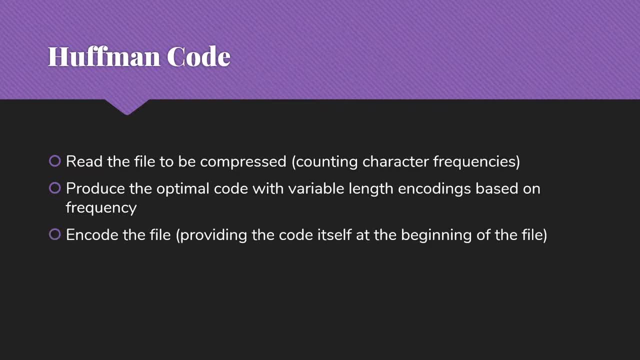 then we're going to encode the file, reading the file again, and provide the code itself at the beginning of the output file, because this code is going to be specific to this particular file, so we do have to also provide the code at the beginning of the file. In general with a file, 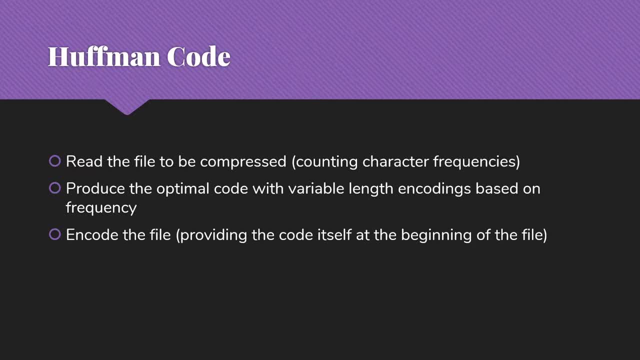 of some length, we will get enough savings that it's worth it, even though we have to include the tree. Then we're going to recreate the code from the information we provided at the beginning of the file and decode the file when we want to decompress it. Now, the key piece of Huffman code is the code tree. 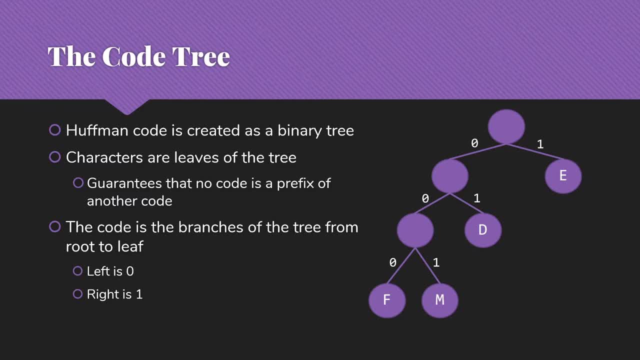 So what we're going to create is actually a binary tree where we have characters of the leaves of the tree. The nice thing about the characters being guaranteed to be leaves is that no code for a given character is a prefix of another code, So we know that if we just go through this code and follow it. 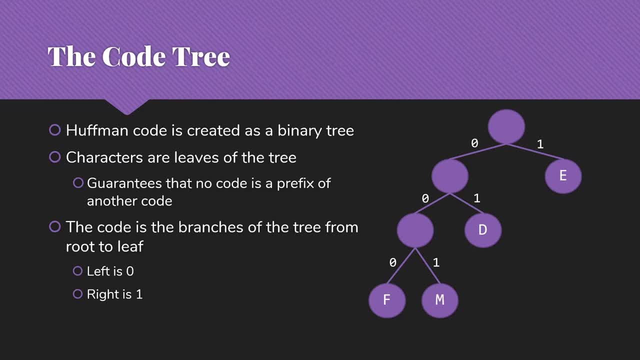 we'll eventually get to the right character. The way we produce the code is if we start at the root and go to a leaf. anytime we go left, we consider that a zero, anytime we go right, we consider that a one. So in this particular case, the code for e would be one. the code for m would be zero, zero, one. 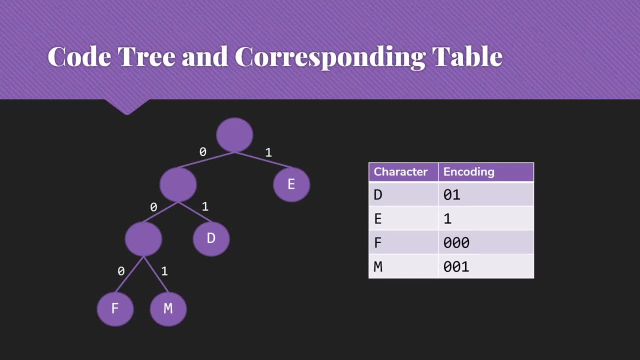 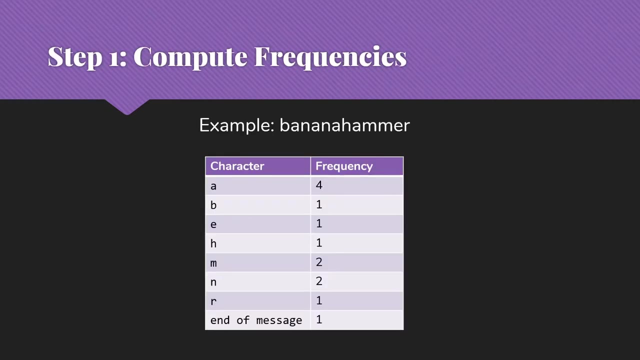 And here is the table that corresponds to this code tree, So we can see the set of bits that we would use to represent each of these characters. So d would be a zero, then a one and f three zeros. So let's see how this works, going through an example. So I have here a simple little message. 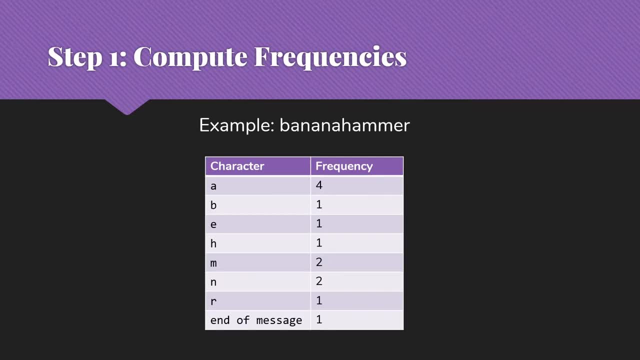 banana hammer, and the first step is going to be to compute the frequencies for all of the characters that appear in our message. So we have four a's, one b, one e, one h, two m's, two n's, one r, And then I've also added an end of message, because we do need some way to recognize that we've hit. 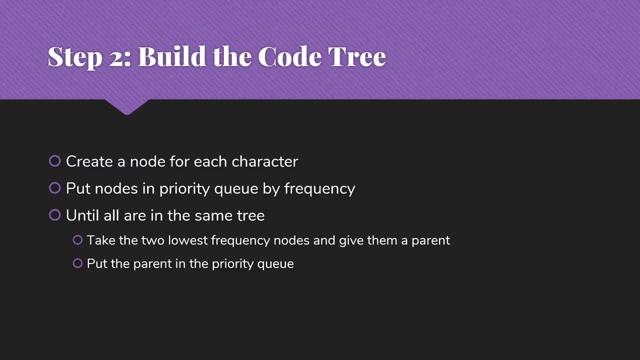 the end of our file. Once I have the frequency table, then I need to actually build my code tree. So the basic idea here is that I'm going to start by creating a node for each character, so I'm basically going to create a forest of trees. 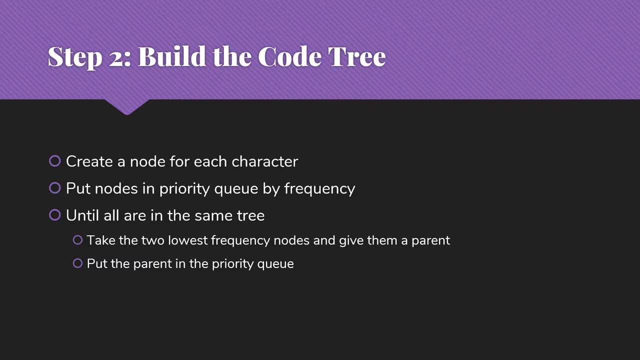 each of which has one character. I'm gonna put the nodes, the roots of all those trees, into a priority queue based on the frequency for that node, which, in this case, is going to be the frequency for the character. Then, as long as I have more than one tree, I'm going to take the two lowest frequency nodes, So the low frequency tree is. what I'm going to say is that I'm going to put these nodes in a priority queue. 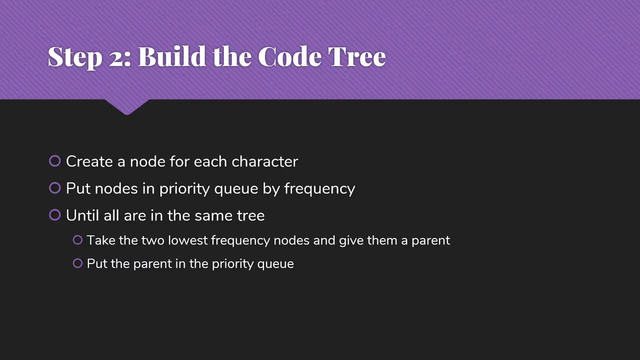 So the lowest frequency trees that I have is going to be the frequency that is going to be used for this character. I have, and I'm going to give them a parent, make a new node adding the two frequencies together for the frequency of this subtree, basically, and then I'm going to put that: 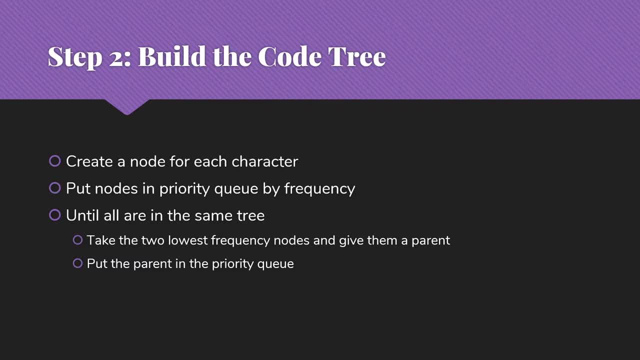 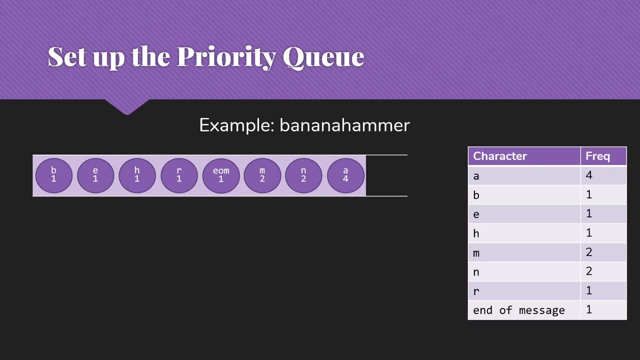 parent back in my priority queue. So let's see what this looks like with our example. First, let's set up our priority queue, So we have our frequency table. We're going to make a node, basically a tree root, for each of these characters and we're 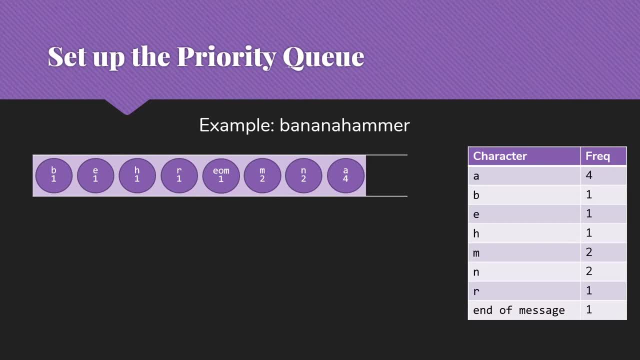 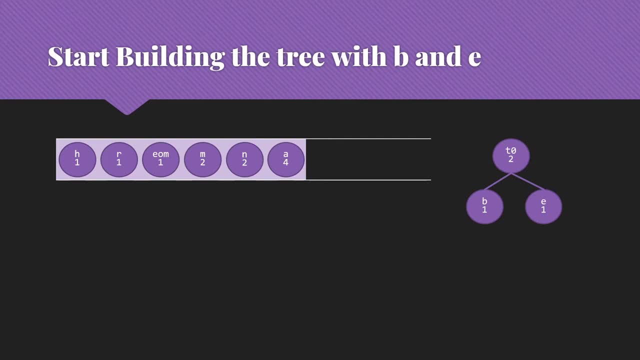 going to put all these things into our priority queue. Once we do that, then of course we're going to go into our loop. So we pull the B and the E off of our priority queue and we create a new node to be the. 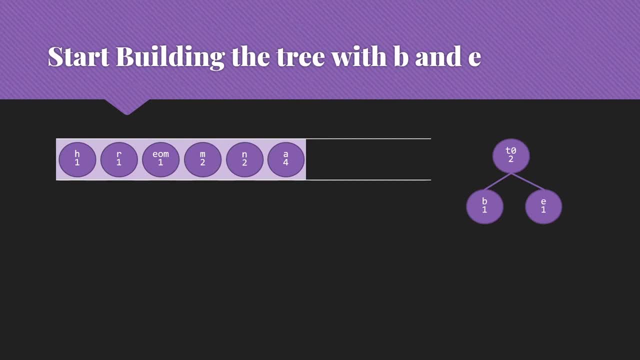 root of a new tree that has the B and the E as subtrees, So its frequency is two. So then we'll add our new node to our priority queue. Then we need to actually take the next pair. So we're going to grab the H and the R, which are the next two items from our priority queue. 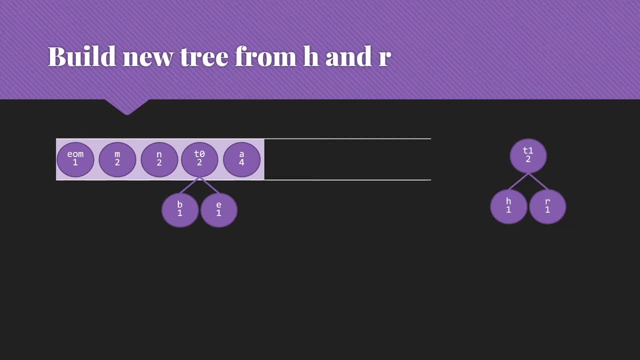 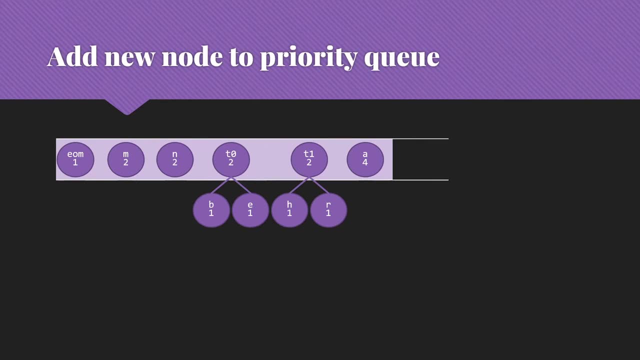 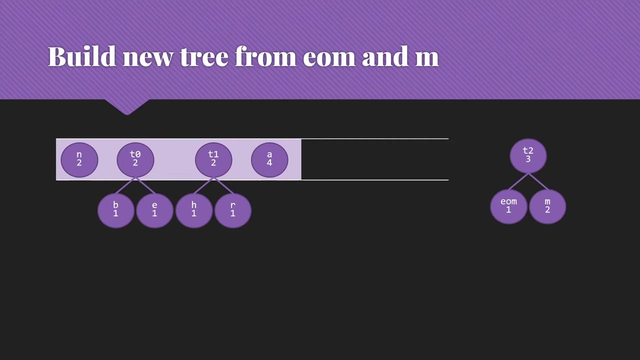 We're going to make their parent T1, which will be also priority 2, and then we will add that into our priority queue. Then we'll go on. We take the end of message And the M. Our new node will have frequency 3.. 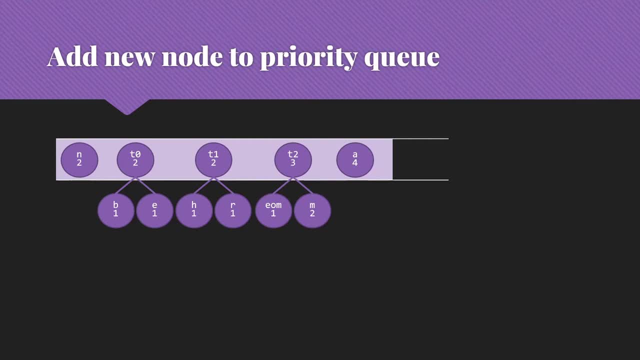 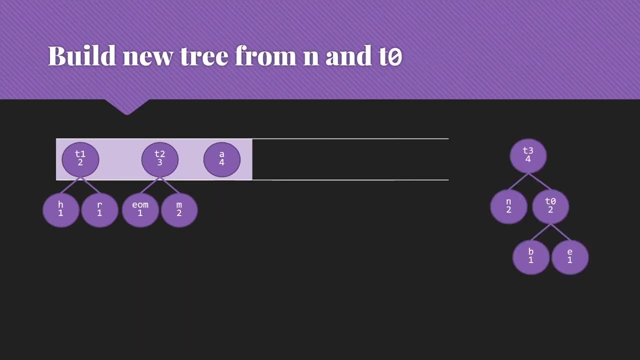 We then will put that into the priority queue. Then we'll take the next two nodes off, the N for 2 and T0, and we'll build T3 to be the root of that tree. Put that in our priority queue, Then we'll grab the next two nodes. 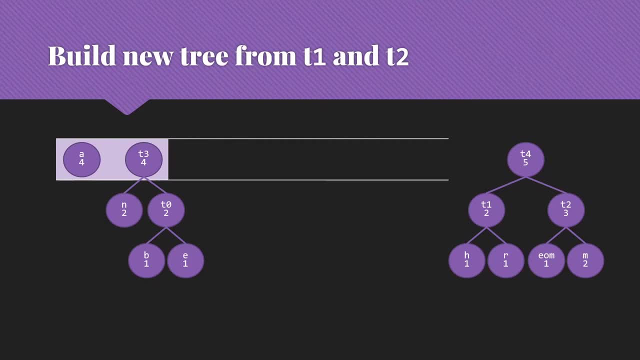 Make T4 to be the root of that tree, Then we'll add that to our priority queue. Make T5 to be the root of that tree. Make T6 to be the root of that tree. Make T7 to be the root of that tree. 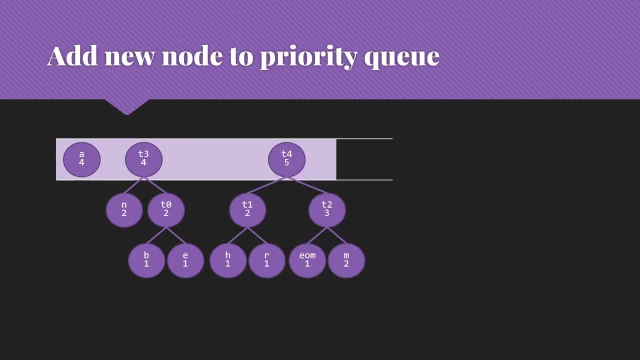 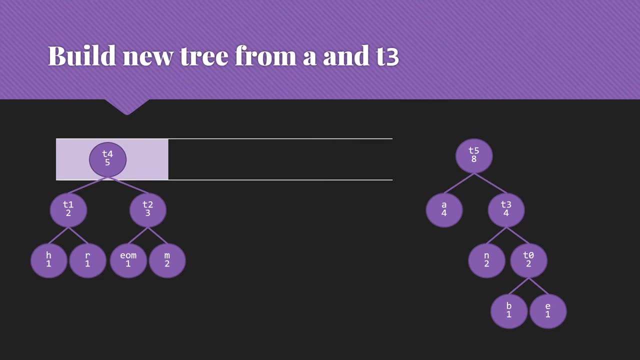 Make T8 to be the root of those two subtrees. that has frequency 5.. So we'll add that to the priority queue. Then we grab the next two, which will be A and T3. We build that node, Then we add the new node to our priority queue. 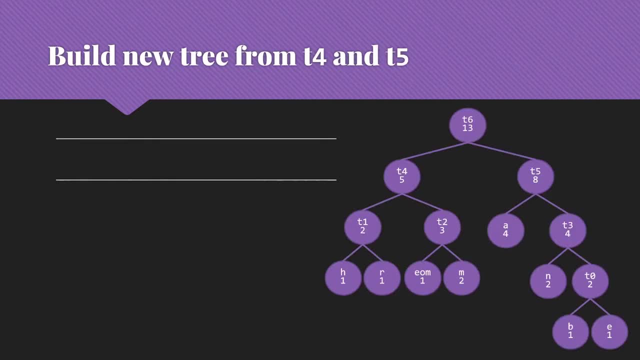 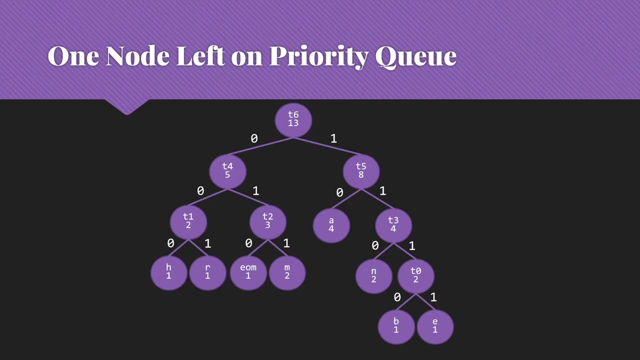 Build the new tree from those two items. Now, at this point we put the node back on the priority queue. It's the only thing left. When we see it's the only one left, then we know we have our final total code tree. 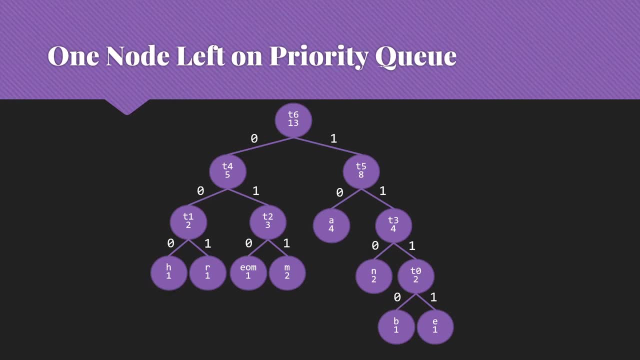 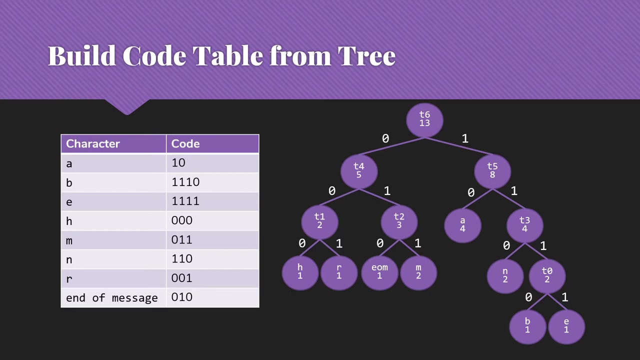 So here is the tree we would build from our message banana hammer. The next step will be to actually create a code table from the tree. So we're going to go through each of our characters and basically go through the tree, do a traversal and find the code. 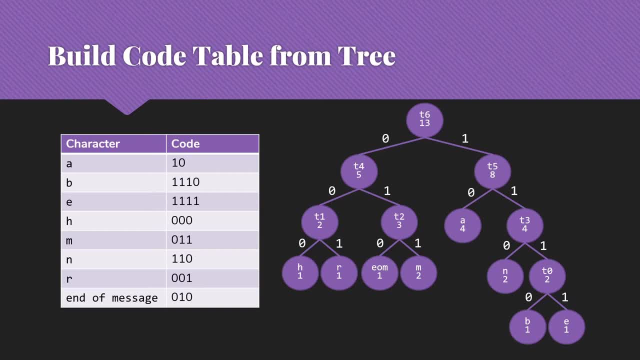 And note for each leaf: this was the code to that character, So we'll end up with A being 1, 0,, B is 1, 1, 1, 0,, E 1, 1, 1, 1,, H 0, 0, 0, 0, and so on. 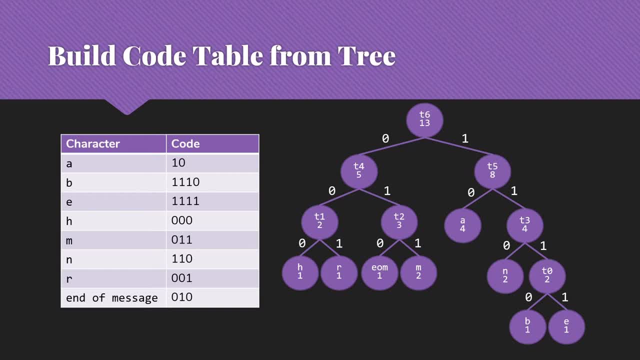 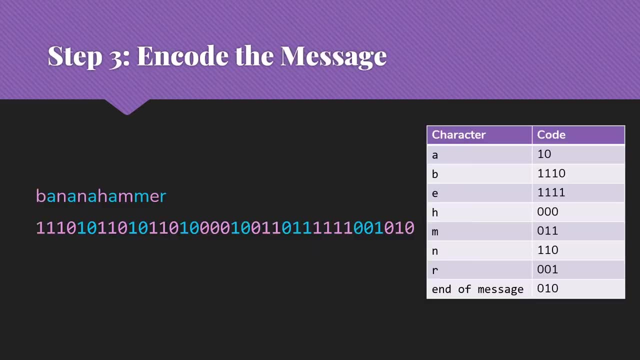 So once we have the code table, it's a fairly easy job to actually encode our message Using the table. So we're going to go through each character of our message and put in the code from the table for that character. So B will be 1, 1, 1, 0, A will be 1, 0, N 1, 1, 0, A 1, 0 again, and so forth through. 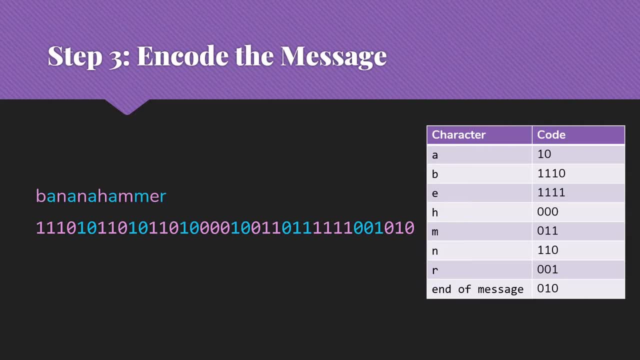 the whole thing And of course, when we get to the end of the message we'll tack on the 0,, 1, 0 for our end of message And then we're going to add in the file the full message character. 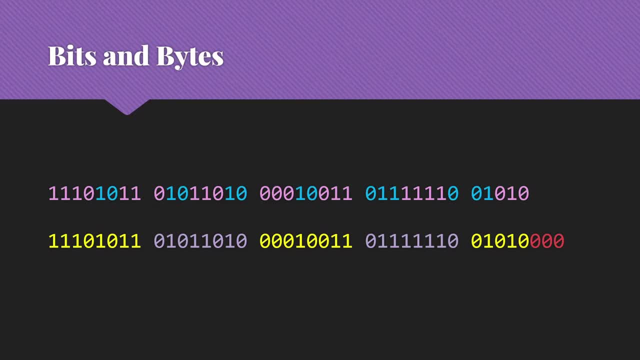 Now we do have one other complication here, and that is that we don't write bits to files. We write bytes to files, So we need to deal with these as bytes. We will need to take our sequence of bits and separate it out into bytes to actually write it. 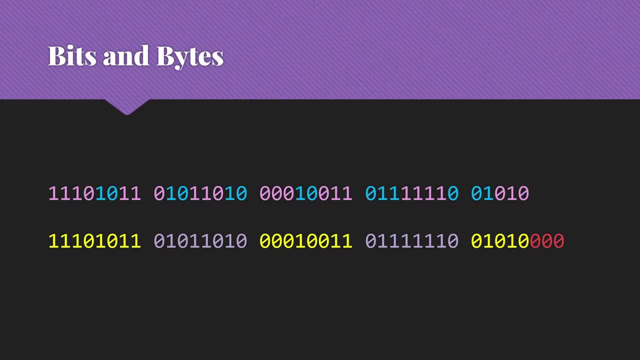 to the file. there are certainly libraries available to help you do that, as well as bit operators that will let you operate on the individual bits of a byte. So we can see here that we're going to take our message, break it up into bytes and write each of those bytes in turn. Now we do have one other. 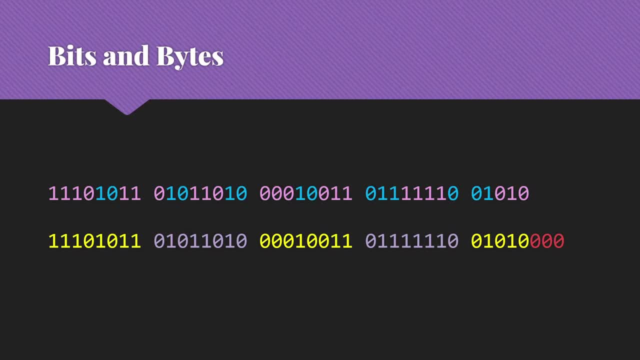 issue, which is that often our messages don't end at an even byte boundary. So what we're going to do is to simply pad that byte on out, Usually with zeros, though it really doesn't matter, because we're never, ever going to look at those bits when we're decoding our message. We're going 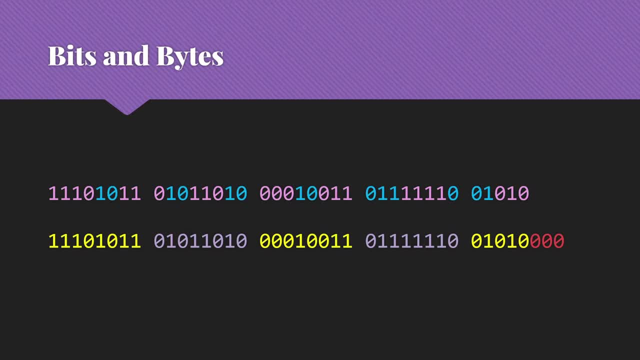 to be able to avoid that because of that end of message character that we included in our code. So at this point we have our message, we can write it out to a file. we then need to deal with what happened to the code, So we can go ahead and decode our message, So we can deal with that. 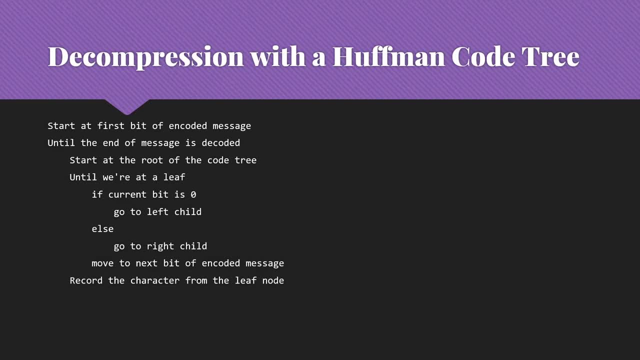 patch. So we're going to decode our message, We're going to build this dialogue and it's going to directly do we do when we get to the other side. so we are going to need to decompress our huffman code tree. so we're first going to need to put information about: here's the structure of the tree. 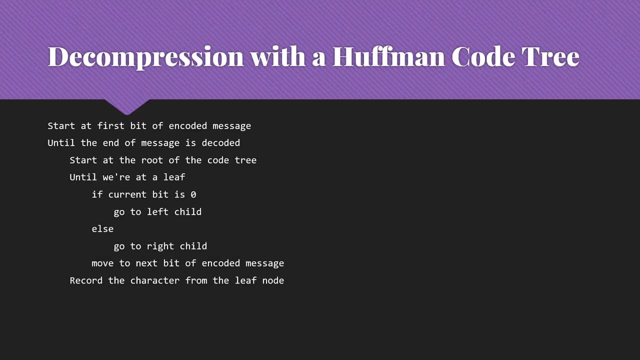 so that we can recreate it on the other end. we always consider that, and when we decide how much we've compressed our message, we always include the amount it took us to express the tree on the other end. now, on this end, we don't bother with the table, we only use the tree that we were using. 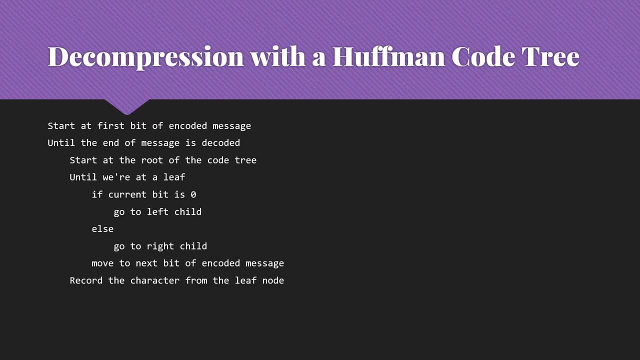 so we're going to do is we're going to start at the first bit of the encoded message. until we have decoded the end of message character, we're going to start at the root of the code tree and until we're at a leaf we're going to. 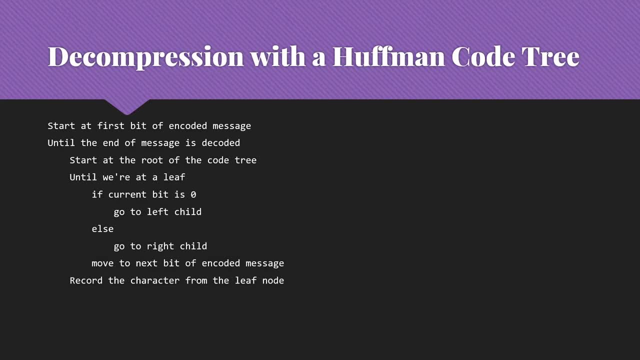 go left if we've got a zero, right if we've got a one, and go to the next bit. when we get to the leaf, we're going to record that character. we've gotten to the end of a code that represented a character, so we say, okay, we've got that character. let's go start over at the root for the 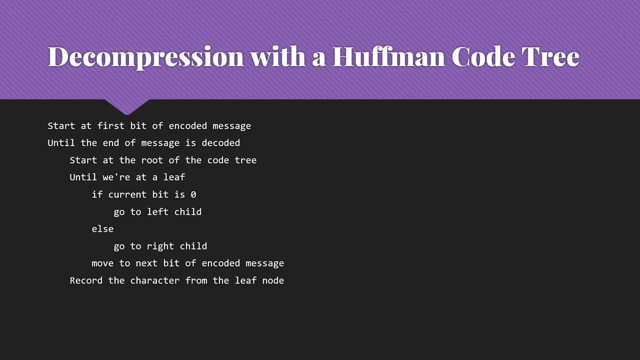 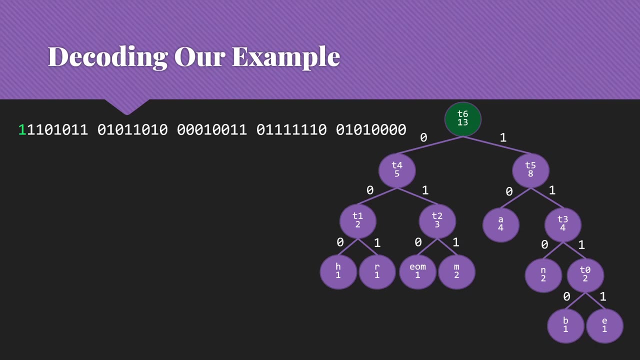 next character. so let's go through the process of actually decoding, decompressing our message that we created. so here we have our message. we're going to start at the first bit and at the root of our code tree, so then we're going to go right because our first bit is a one. then we'll go right again because we 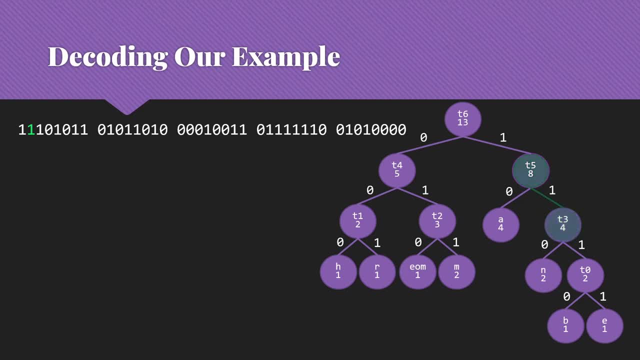 have another one. then, of course, we have another one, so we go right again. and then, finally, we're going to get to a zero, so we'll head left and we find the b, so we've got our first character. now we need to start over at our root. we're at a one again, so we head right, but this time 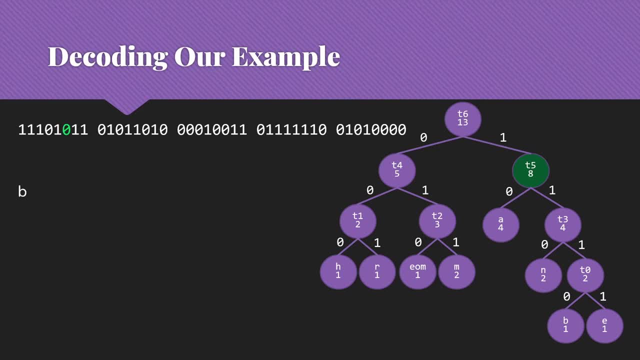 we have a zero, so we will now head left and we get our a. that gets us another character. so now we need to go back to our root. we're going to head right and then we will see that we need to head right again. then, moving on from t3, we have a zero, so we're going to head left. now to the in. 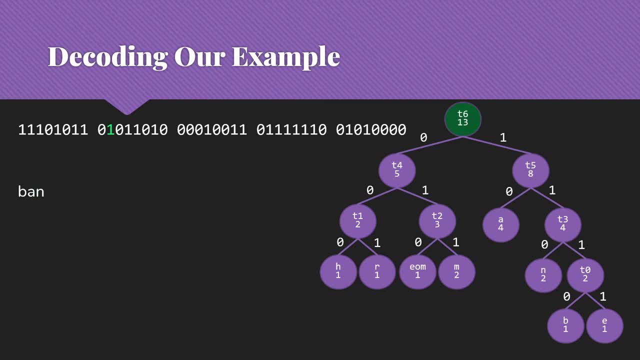 that gave us a new character. so our next step is to start at the root, where we head right again and then we're going to head left and that's going to get us another a. so back to the root again. we're going left, we're going right again and we can see that we're going to head right. 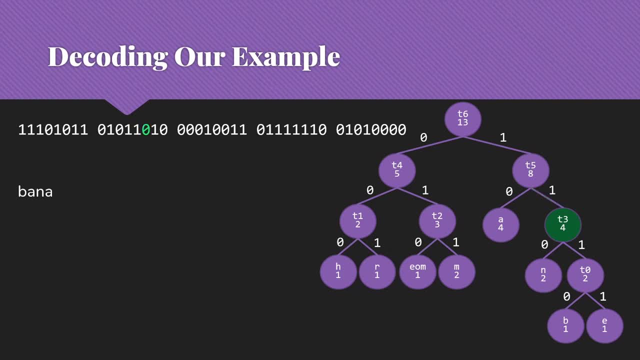 and then our next character is a zero, so we're going to find ourselves with another in, so that means that we're going to head left, then we're headed right, and then we can see that we're going to go left and pick up the next day. 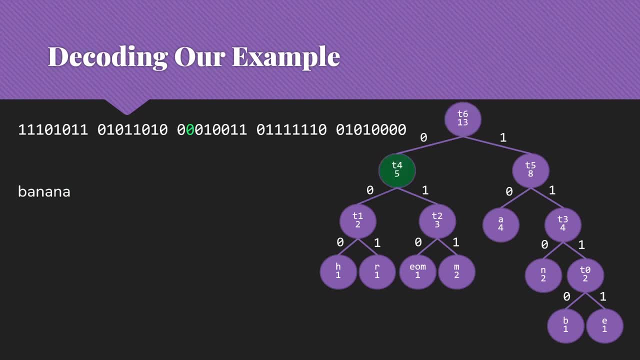 then the next time we're going to go left, left again, and then left again, and then left again, which will get us our h. Now we need to start back at the root. so we're headed right And then we're headed left and we're going to pick up that next a. 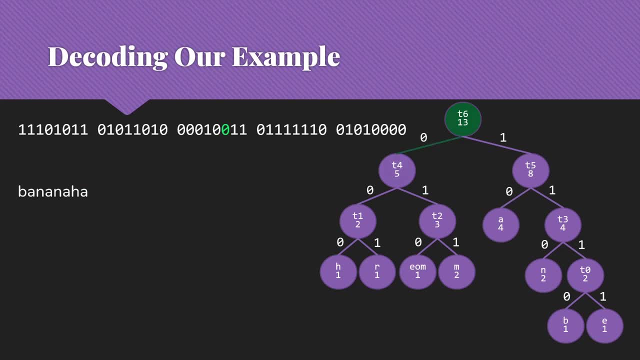 Then we head left again, so we're at t4.. This time we're headed right from t4 to t2, and then right again, where we're going to find an m, And we do actually the exact same thing: We're going to head left. 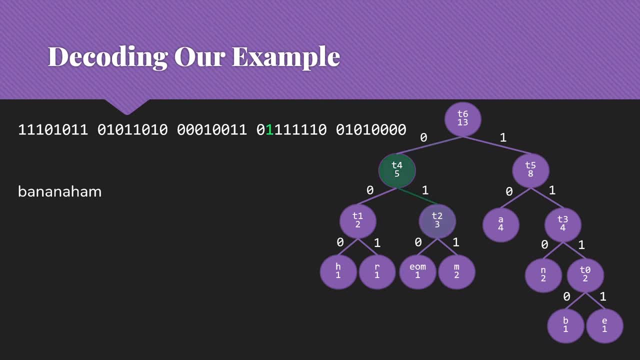 We're going to head right. We're going to head right again and get ourselves another m. In this next case, we've got a right for the 1.. We have another right with another 1.. Then we have another right. 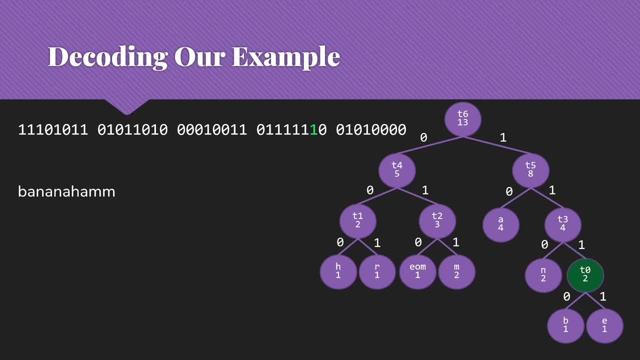 And yet another right where we're going to find our e. We're going to head left to t4.. We're going to head left again to t1.. Then we're going to head right and pick up that r. Then we're back up at the root with the left. so we're back over to t4..